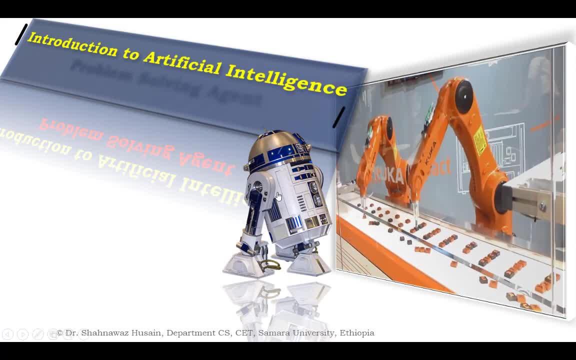 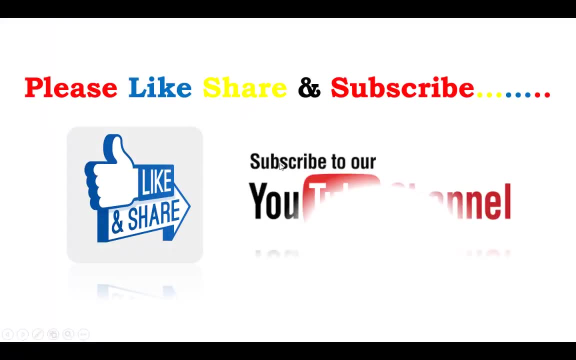 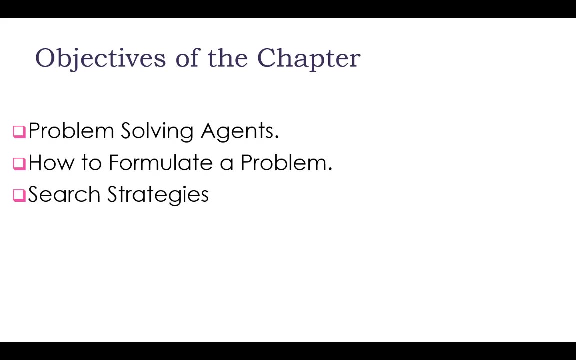 Welcome back to the tutorial of artificial intelligence. We are discussing about problem solving agent. Please like, share and subscribe the channel to show your support. These are the following objectives of the chapter. If you remember in the previous section what we discussed, we discussed about the introduction of the artificial intelligence. 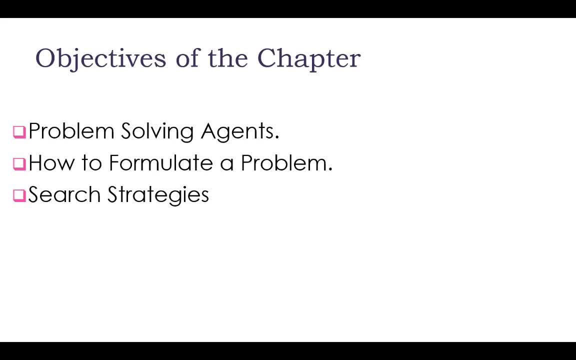 That is, we have defined the boundaries of the artificial intelligence and how one can define the definition of the artificial intelligence. And further, we discussed about the foundation of the artificial intelligence, That is, how many disciplines and branches has contributed towards the development of the AI. 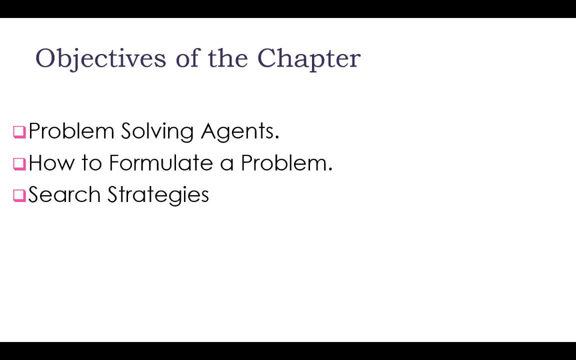 And the next thing: we discussed about the generation and history of the AI, about the evolution of the AI up to the current development of the AI. Next, we discussed about the history and generation of the AI and the possible application of the AI we have discussed in the chapter 1.. 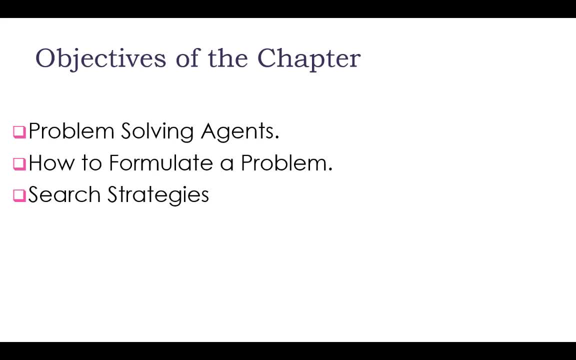 In the further chapter that is related to the intelligence, We discussed about the type of the agent and how can. what is the intelligent agent? why we are using the term agent. We are using the term agent because anything which is doing its job in the intelligent way it is called as intelligent agent. 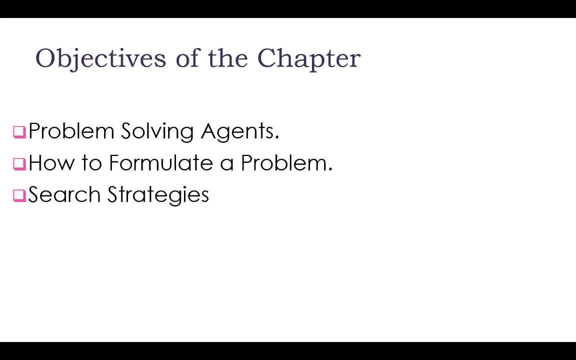 So in intelligent agent or according to the definition of the intelligent agent also, the human is also considered as one agent, Robots- they are also considered as one agent and the software is also considered as one agent. And the types of the agent we have discussed, that is simple reflex model, model based agent, goal based agent or utility based agent. 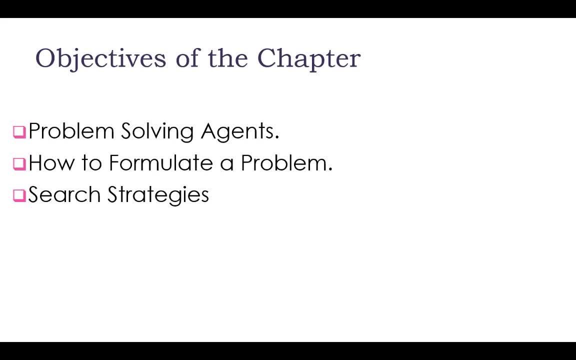 And also we have discussed about the learning agent And in the same section we have discussed about the architecture or structure of the AI agents We have discussed, that is, the agent can be defined as agent program plus its architecture. Remember that as an AI. 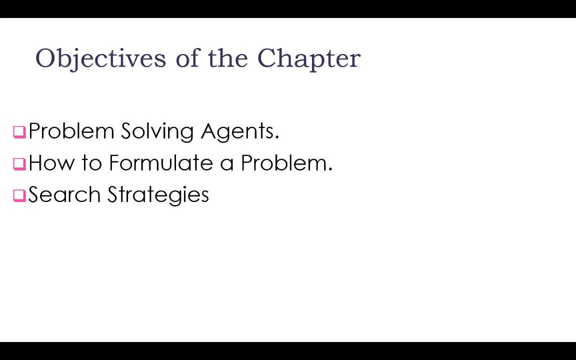 Programmer. we need to focus upon the agent program. we are not going to focus upon the robotics. maybe it is part of the AI, but it is. we are not focusing this time on the architecture of the agent. we are only focusing on the agent programs, and these programs we have discussed already: simple reflex model, model based agent, goal based agent and utility based agent, and also the learning agent. 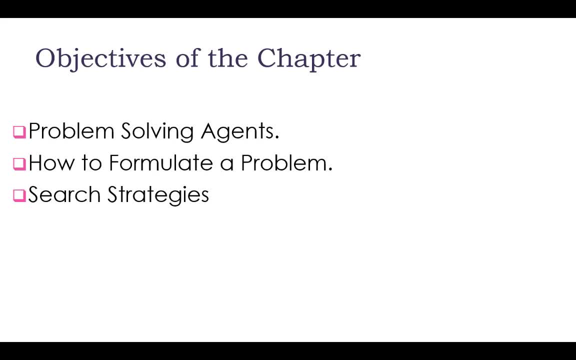 So these four or five, actually learning agent is not the type of the agent it is So for this chapter. these are the three definitions or three objectives we are having. we will discuss about the problem solving agent And the third one, the learning agent. 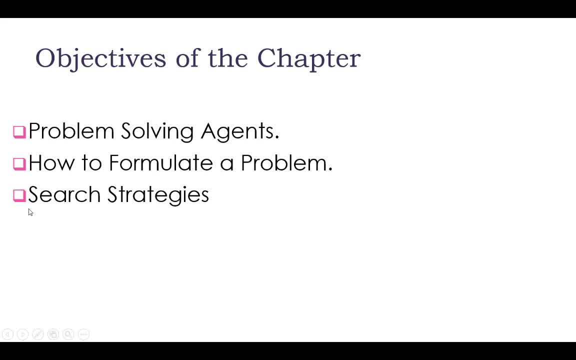 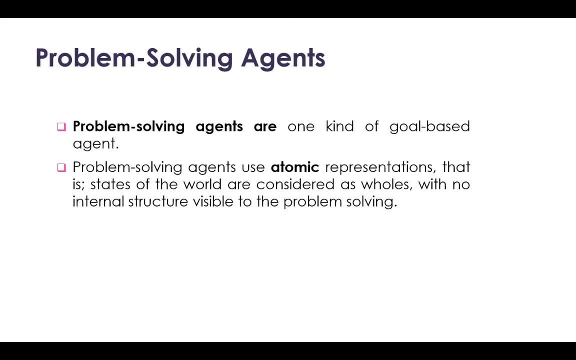 we will discuss how to formulate the problem and we will discuss various search strategies related to find the solution of the given problem. this is problem-solving agent. how can one define the problem-solving agent? if you remember, in the previous chapter we discussed about the goal base agent. what 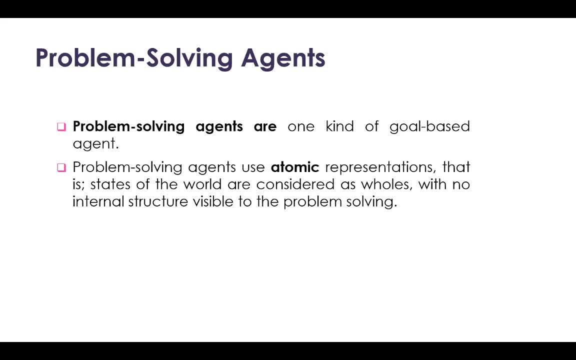 is goal base agent. goal base agent is the agent which is having a specific goal to reach the example for this one we have discussed that suppose that a taxi driver it is coming to the crossing and it has the various option on its hand that it it can go straight, it it is having the option take the left turn it. 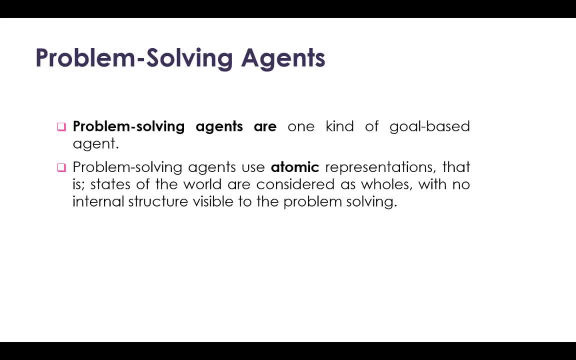 is having the option to take the right turn, or it can make the u-turn also. that is also possible. so in that case, which option the agent should select? it is only possible or it is possible to make. the u-turn is simplified for the agent if the goal is given to the agent, that is, the taxi. 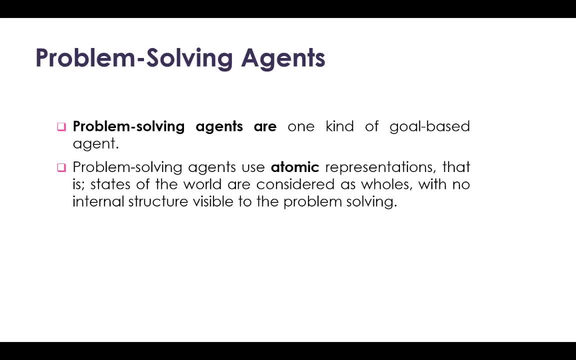 driver has to reach to this particular position or this particular location. so it will simplify the problem and the agent will have the option to select which direction. if I will select straight, in which direction I will reach? if I will select the left or I will select the right, which direction will? 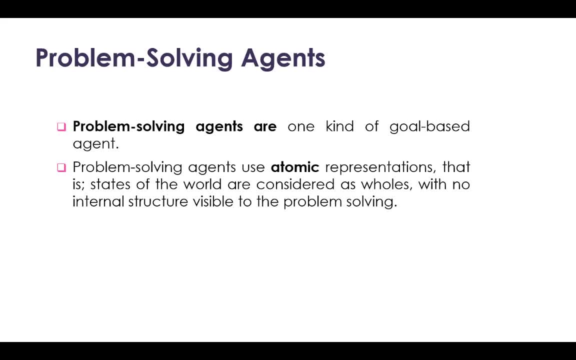 give the way to reach to the goal. so this is goal base agent and this is a very broad category of the agent. that is goal base agent, the problem-solving agent, problem-solving agent is one kind of the goal base agent. remember that this is only one kind of the agent, it is not the. 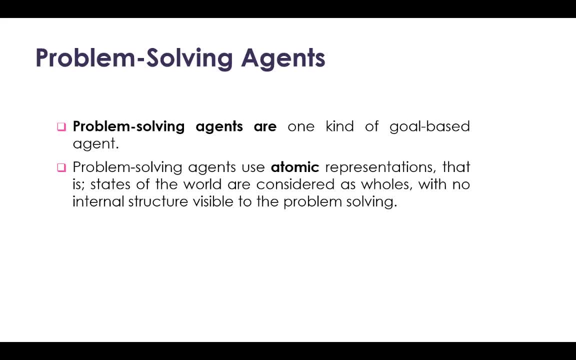 complete definition of the goal base agent: problem-solving agent. mostly it is this kind of the agents. they are used to solve the specific problem. based upon the code we are, we are searching the solution for the given problems and the related object, without, though I already have the universities and libraries. 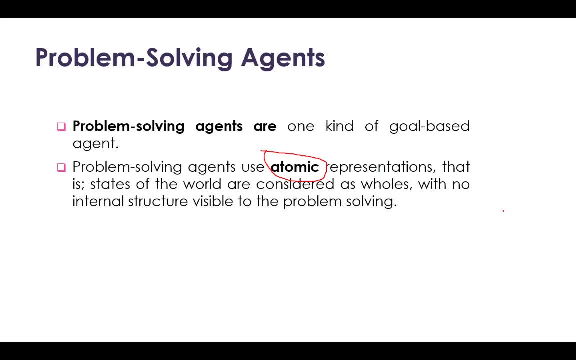 now the problem-solving agent. we are saying that, if you see here that is saying that it is using an atomic representation. what is atomic representation? when we are saying that atomic representation is meaning is that the state of the world is considered as whole. what is this meaning? how can we? 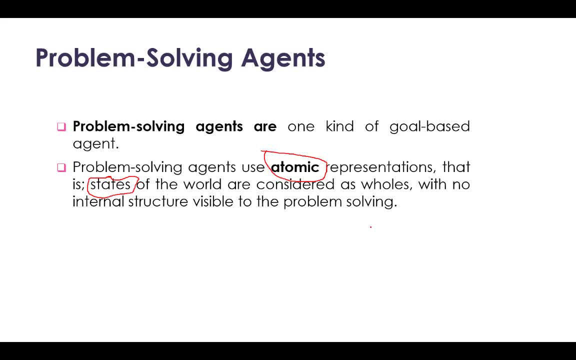 define it in simple that suppose that a only the taxi driver single on it on the road. no other taxi driver or its competitors are on the road. so it is moving as it wants. but the real world scenario may be different. maybe it is having that different hurdles different. 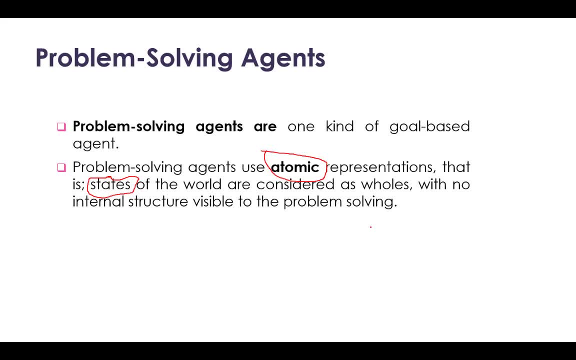 signals and various hidden hurdles are there. so in the problem-solving agent, the atomic structure is given a pot, atomic representation is given to us, that is, we are having only the top view, that is, the states are given, that is, if the agent will move from this state to this state, it will reach to this. 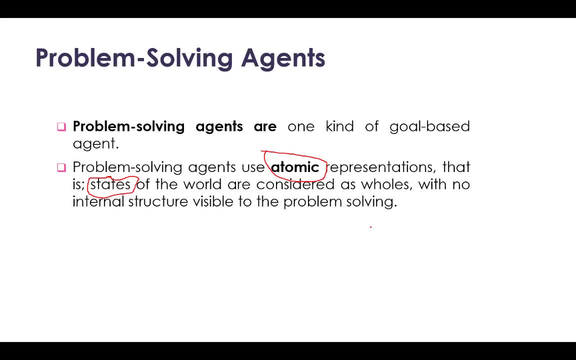 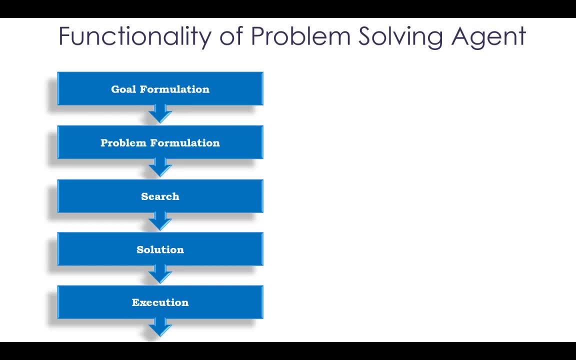 particular state, but the hidden hurdles are not defined here. this is the functionality of the problem-solving agent, how it is searching the solution for the given problem. if you will see, it is a five step job for the problem-solving agent. it is having goal formulation, problem formulation, search solution and. 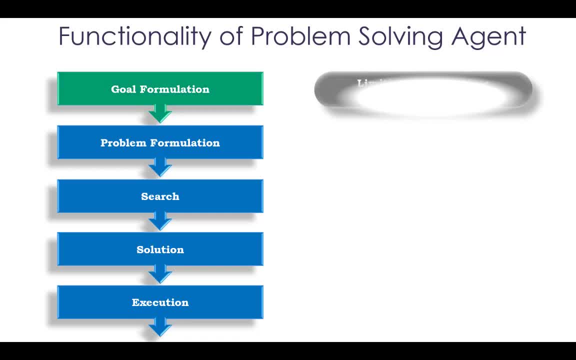 execution of the solution. so the first one is about the goal formulation. what is goal formulation actually? goal formulation is very easy task for the agent because goal is given to the agent, that is, he needs to reach to the particular state or particular position. this is the your goal. so when the agent 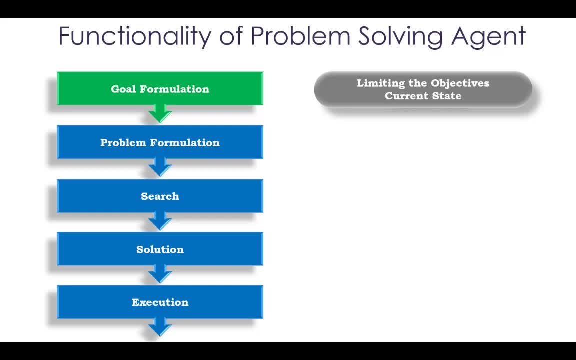 is coming to the goal formulation, it will in. the objective is to limit the reboot ofars are exposed to the objective. the aim of the goal formulation is to limit the objects. I suppose that if the agent is having multiple goals so it will be very difficult for the時間 to search the 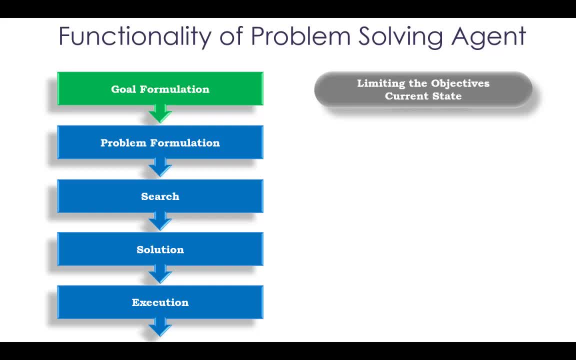 solution, so limiting the objectives. it will decide a specific objective and what it will get: an. it will be written the current state also, that is the initial date of the agent. the next step: you are having the current state as well as the objective, the specific objective. the problem formulation will calculate. 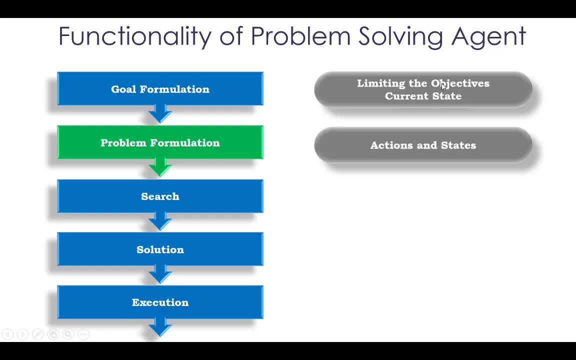 the actions and the possible states, based upon the current state and based upon the objective. so it will return. problem formulation, will return the action in its state and remember that problem formulation is the most important part of the problem-solving agent. because goal formulation it is the simplest task, because we need to select one goal: what is our goal? but when we 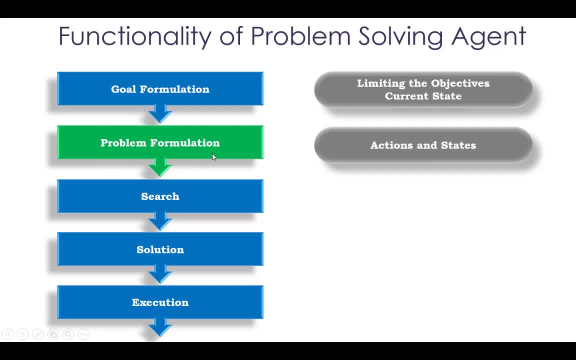 are talking about the problem formulation, because in the problem formulation the problem may be given to us in the story language or maybe some fictitious story, and if you are not able to convert this problem into the formal system you cannot reach to the goal. so problem formulation is very 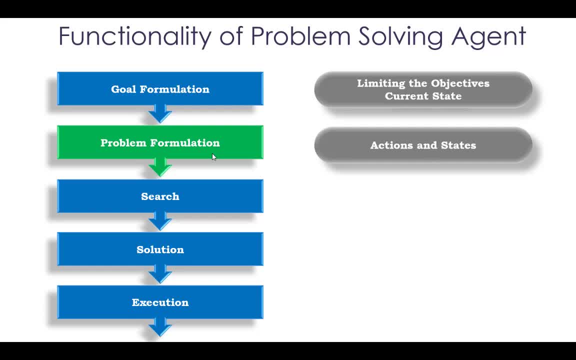 important part. we are going to convert the step-by-step solution, or you can say that a formal step. we are converting the problem from the problem form to the problem form. story type story like problem story. like definition. the next one is about the search, what it will do. the search will identify the possible sequences of the action to reach the 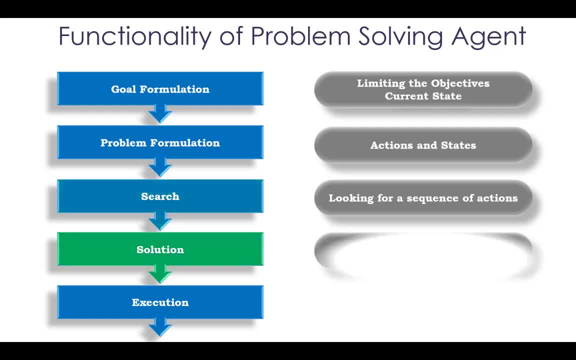 goal from the current state. next thing is about the solution. what is solution actually for this particular step? we need to search the algorithm. which algorithm- searching algorithm- is best suited for our problem and based upon that one, this search algorithm will take the problem as the input and it will return the solution. remember that we need to reach to the particular goal. 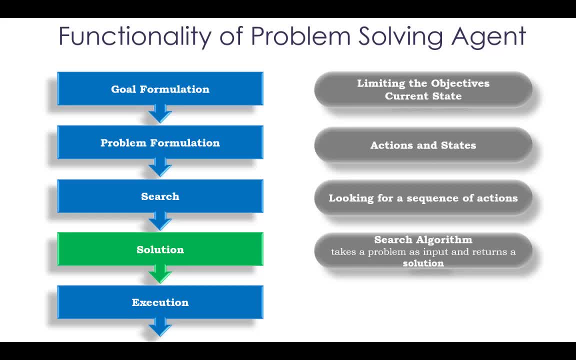 so, as an input, it will take the problem and goal will be the output and it will reach to the goal. and this search algorithm, multiple solutions for you, but remember that which is the optimal solution. it is best and our objective or the best searching algorithm is one which is providing the best solution or optimal solution. when you get the optimal, 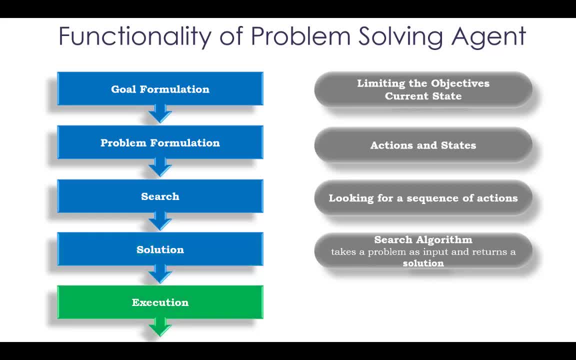 solution from the searching algorithm. this is the task of the problem-solving agent. to execute the actions, that is, the series of the equations or the sequences of action from the current state to the goal, is state now, problem formulation. what in the previous slide will be shown in the next slide? 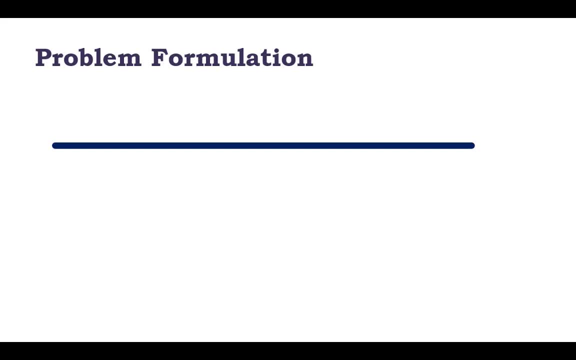 have discussed, that is, problem formulation is very important part because it is if you are able to convert the problem into the formal language, that is, in terms of the mathematics. it is easy to identify the solution if the problem you are not able to convert into the formal step. 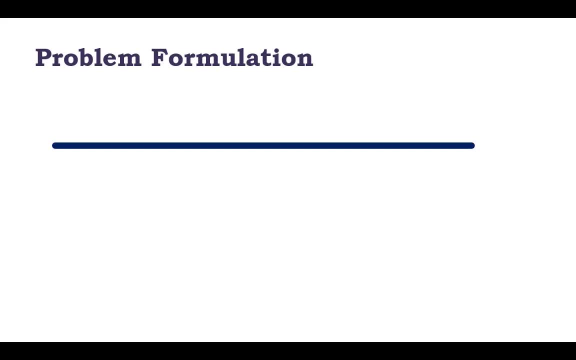 you cannot get the solution. remember one this thing: it problem formulation is actually five step job and we will discuss all the five step in detail. the very first step: we are saying that that is the initial state, initial state of the problem, and you will get it from the 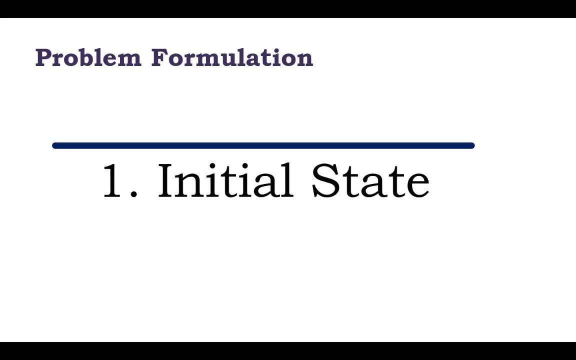 goal formulation, what is the goal formulation, whole formulation will give you the initial state or the current state. the second thing is that a specific object, your specific goal, when you identify the initial state or the current state of the agent, the second step is to search the action, that is, if i am on the particular situation. 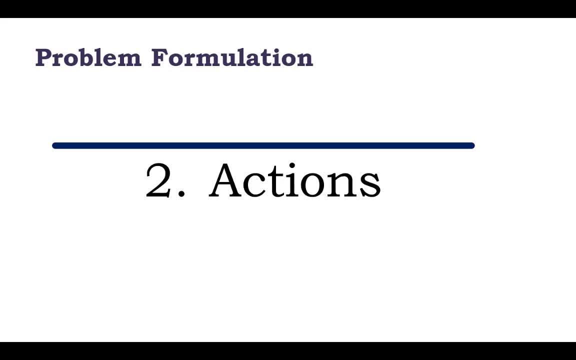 or particular state. what are the options or actions are available on my hand? and the third step is about the transition model. what is transition model? transition model is that suppose that if i am standing on the current situation, in that situation i am having three or four option. so if i will select the one action, then what will be my next state if i 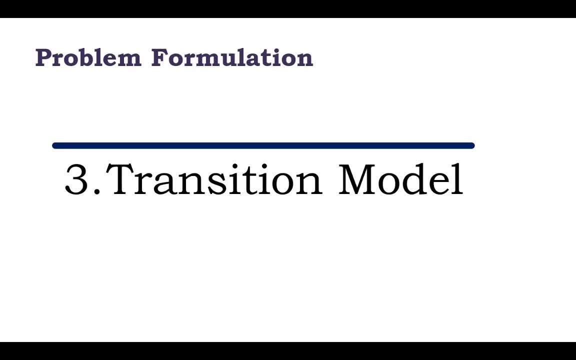 will select the second action, what will be my next state? if i will select the third action, what will be my state? so transition model will define, that is, from the current state to the action and what action will generate for you. the fourth one is about the goal test. what is goal test? goal test i. 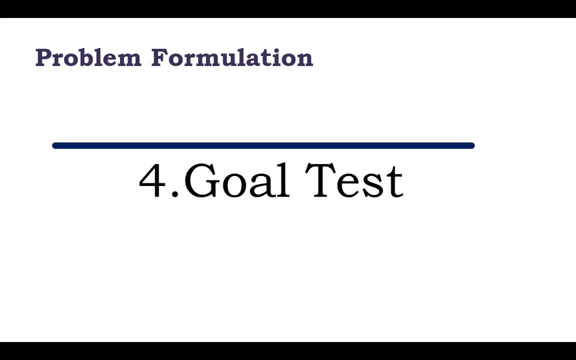 will tell you about that later, but actually after taking the transition model, that is, if you are going, you are going to select a particular action and you are reaching to the certain state. at that time you need to compare your goal with the that state, that is, you, the agent, is reached to the goal. 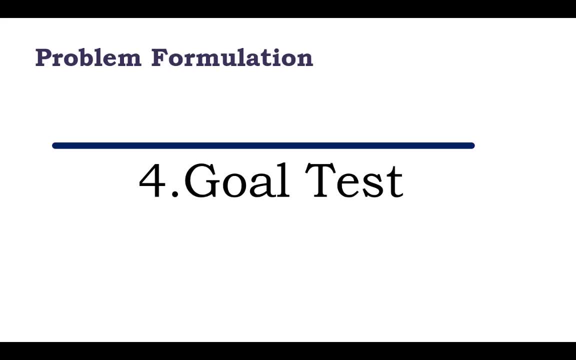 or not. if it is not reached to the goal, it can take the further action. otherwise, if the goal is reached, it will declare that i reach to the goal. so goal test is necessary after the transition model, each transition model. it will check the goal, that is, the agent is reached to the goal or not. the next: 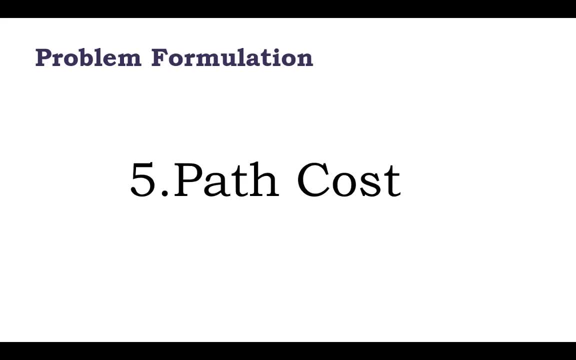 step. we are calling it path cost. what is path cost actually? if i select, if i am on the current action, that is, the agent is on the current state it is, it is selecting the particular action and then it is reaching to the particular state. so what is the total cost during this travel or during this? 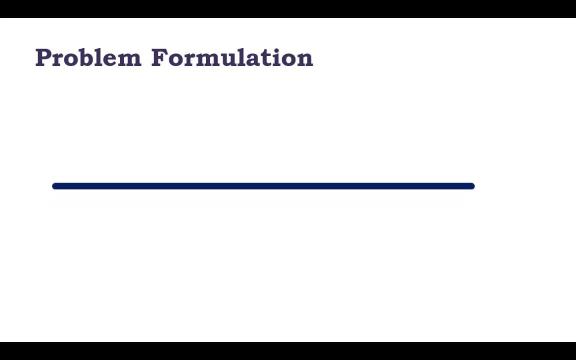 action. the last step is about the path cost. path cost is not the necessary step for the problem formulation, but in another way, it is necessary because path cost will only decide the optimal solution. and what is path cost? we need to check the path cost each and every time, that is. 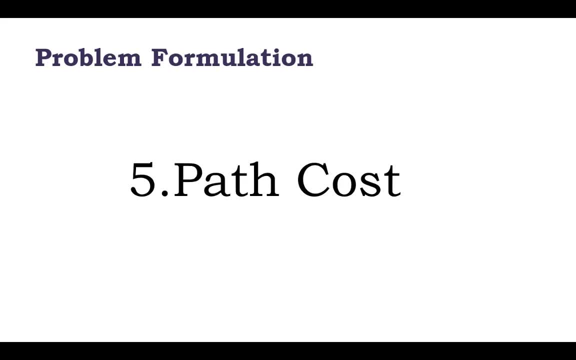 from the current state to the next action and what is the next state during the this transition? what is the path cost? path cost may be in terms of the kilometer, meter or in terms of some unit. may be a resource cost also or cpu cycle also. we need to define. 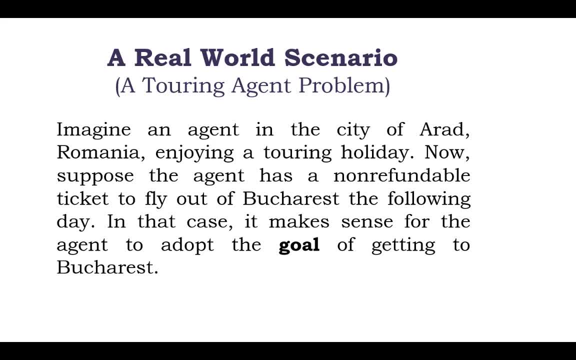 now what we discussed about the problem formulation. we will solve this problem formulation with the help of a real world scenario. look here the scenario is given for the touring agent. This is the touring agent problem and this problem it is given in the terms of the story. The story, if we will read, we are saying that: imagine we are having the assumption that the agent or touring agent, it is in the city of the Arad and Arad is a city of Romania state and the agent is enjoying a touring holiday. 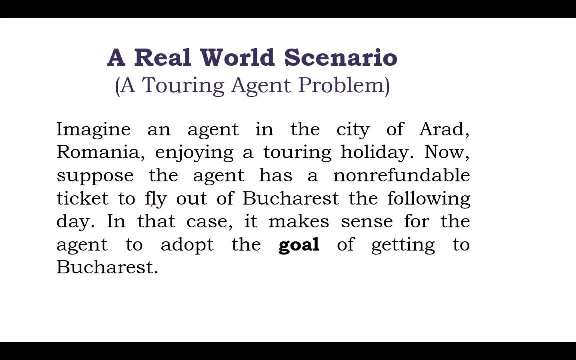 So now suppose the agent has a non-refundable ticket to fly out of Bucharest the following day. In that case it makes the sense for the agent to adopt the goal of getting to Bucharest. So remember that here the goal formulation is very easy, That is, we need to go to the Bucharest at any cost. This is the goal given to us. but problem formulation, Problem formulation: from the goal formulation we are getting that the agent is enjoying a touring holiday. 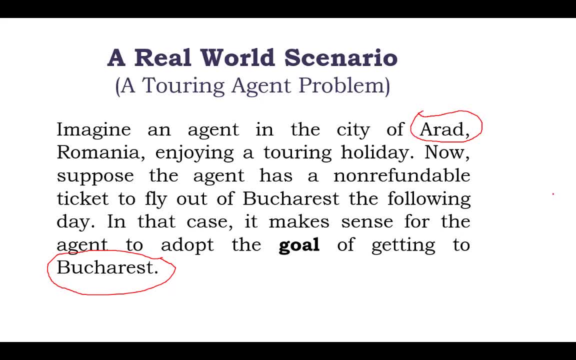 The agent is on the current situation, that is, Arad of Romania state. From this to this agent needs to reach. So to reach up to this point, agent needs to formulate the problem. then only it can reach to the Bucharest. Remember that from Arad to Bucharest there are various paths. So we need to convert this touring problem in terms of the problem formulation. 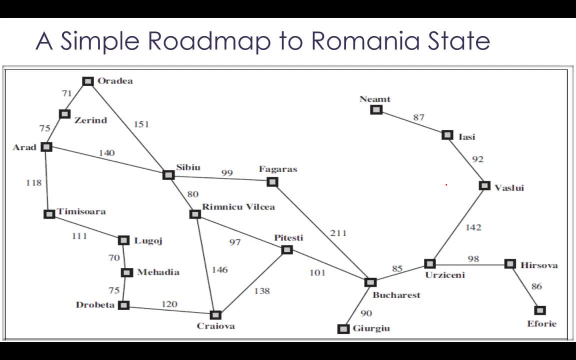 This is the simple road map to the Romania state. From this figure we can observe that we are having approximately 20 cities of Romania and this is the current location of the agent. that is Arad, and this is the goal of the agent: to reach the Bucharest because it is having the flight from this place, and to reach from Arad to Bucharest, it is having multiple options. 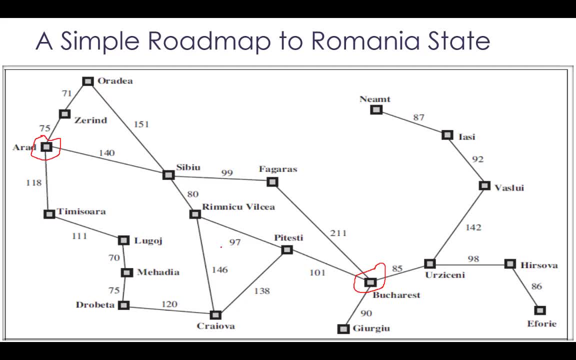 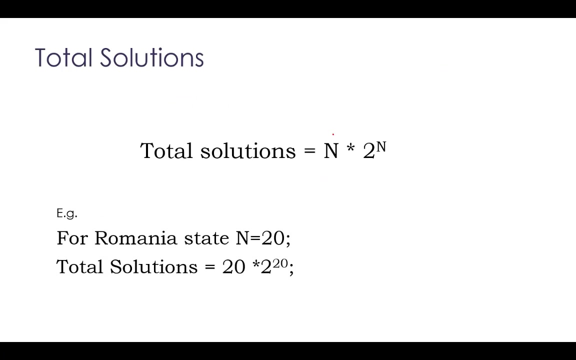 It can travel with multiple directions, But our objective is to identify the optimal solution. Remember that the total solution, how many total solution we can generate from this scenario. The example: for this example, we are having total 20 cities for the Romania state. So the total solution we can generate n into 2 to the power. n n stands for the state, that is, total states available. 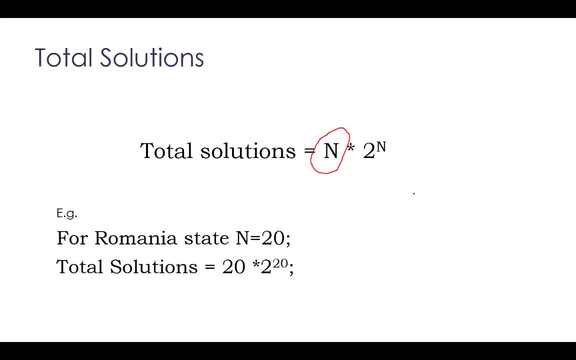 And solution We can generate in two ways. one is proactive solutions. proactive solution meaning is that all the solution we should generate first and kept inside the memory, and the second is reactive. that is what is. if something is action is needed, at that time we need to select. 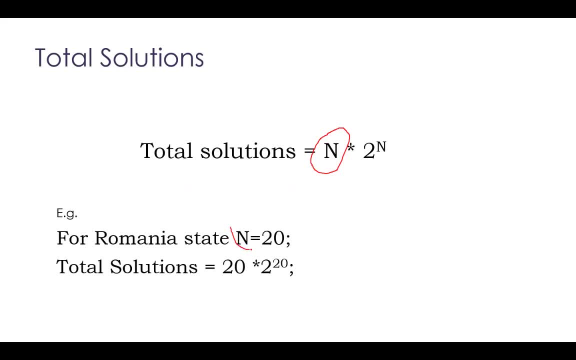 So, if you will see, if we are having the only 20 state, that is, 20 cities, if you are having the total solution we can generate up to these values, that is, 20, to the power, 20 solutions are possible for this situation, For this current situation, that is, we are having 20 cities of the Romania state. 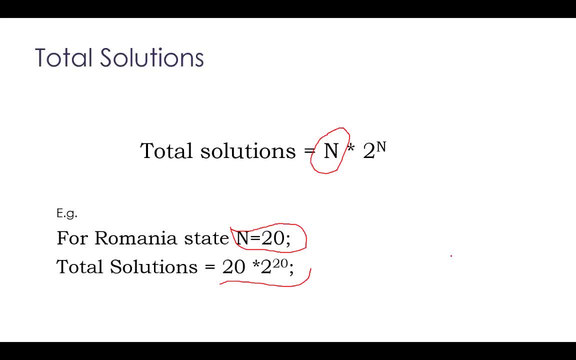 So this is the basic example. you can imagine the complexity, or image space complexity for this kind of the situation. So we are not focusing upon the proactive solutions. we need to search the reactive solution, that is when the solution is needed. at that time we need to execute the search algorithm to identify the optimal solution. 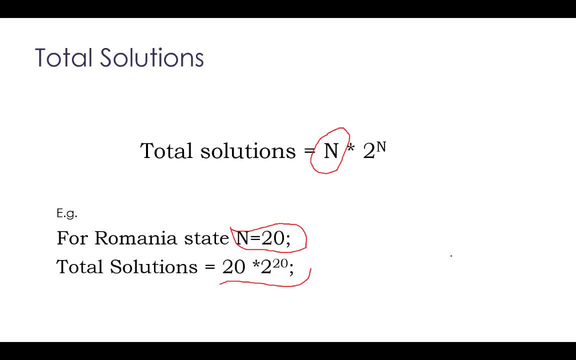 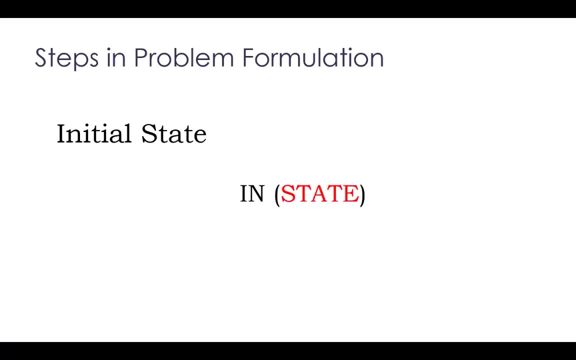 So It is not A Good Suggestion to store all the possible solution. we need to focus only upon the best solution. So now let us start the problem Formulation, which is very important part. the first step is initially state. Now we can write this thing in terms of the state, that is, initially state of the current situation. 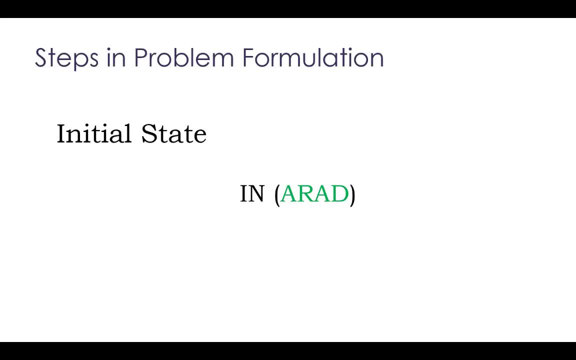 For our problem. The initial state is actually RR, So the agent initially state is given to us RR. Now the second step is we need to take the action, The action state, that is, if I am on the particular state, that is the current state. 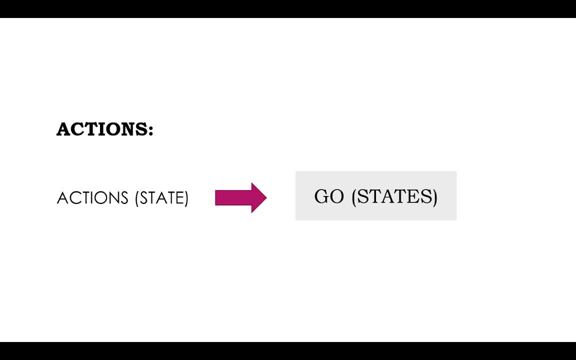 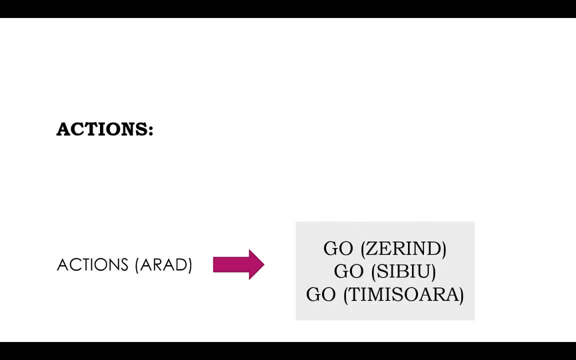 It is having the three option. If you will see from the previous figure, it is given that from RR it is having the three option. The agent can travel to the Zerim, It can travel to the Cebu, It can travel to the through the Timisoara. 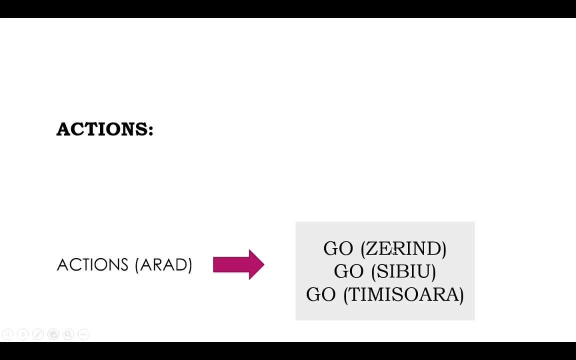 So agent, if it is standing on the RR, it is having the three possible solution or three possible actions which which agent can take. The second, the third one, is that The third step is about the transition model. Transition model meaning is that this is the current state. 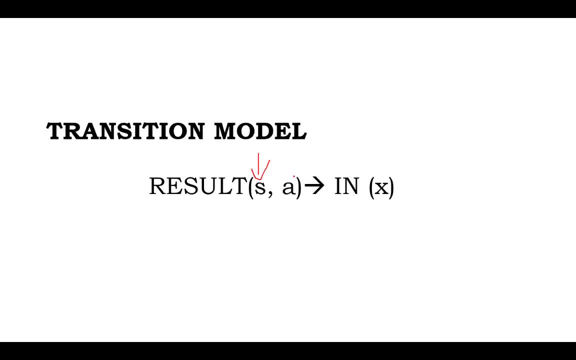 As you stand for, the current state, that is, agent is on the current state and A is the action. that is, if agent will take particular action, What will be the next state? that is, the future state of the agent. This is transition model. that is, transition of the agent. 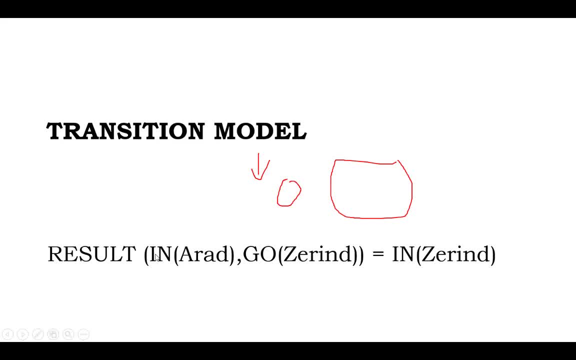 So if you will see for us, if the agent is in RR And if it is taking the action to go Zerim, Then the output is on our hand, is Zerim. That is, the next state will become the Zerim. 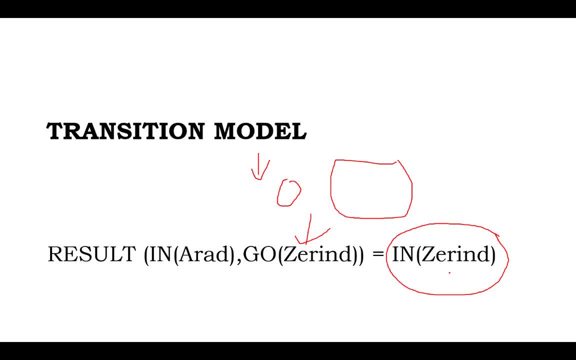 So in this way we are having multiple option, the transition model for us. The next step We need to take for the we need to check for the goal test, that is, if, after the transition model, the agent is coming to the some initial state. OK, 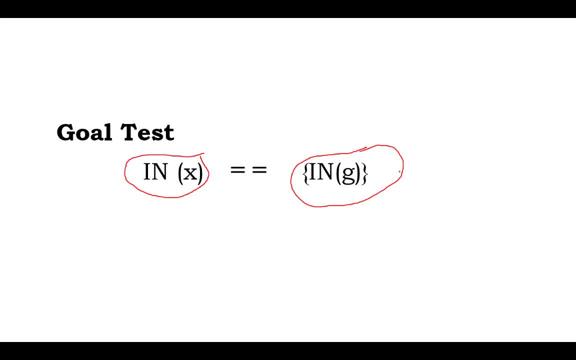 And we need to compare with the goal test, that is, the next state which the transition model is generating is equal to the goal state or not. So if you will see, for our case, Bucharest Our Goal. So each and every time we need to compare with the Bucharest, that is, agent is reached to the Bucharest or not. 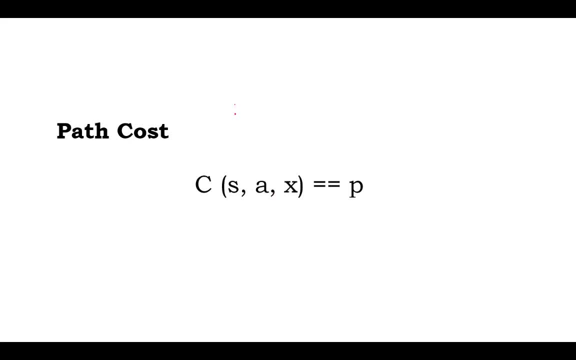 The next step is about the path cost. path cost, if you will see, this is the current state, This is the action. if I will take the particular action and it is reaching to the next state, then what is the path cost? path cost maybe kilometers, centimeter or some definite unit. 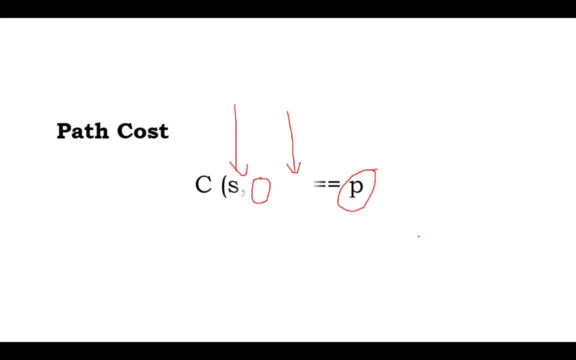 Maybe it is CPU resource cycle or some other thing. So for the current Current situation, if you will see, the agent is on the RR and if it is taking the action to go there in and the transition model is saying that it will reach to the Zerind only so the path cost is generated. 75. the unit is not defined here. you can define the unit as per your requirement. 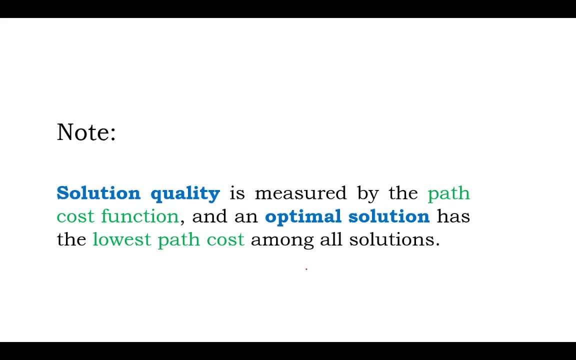 So remember that path cost will give you the solution quality. it will give you the solution Quality. maybe you will generate the multiple solution, or unlimited solution, or limited solution, whatever the situation of the problem, but the path cost, path cost function, the last function. with the help of the last function you can decide the optimal solution. which one is the optimal solution and optimal solution? you can say that the lowest path cost function.